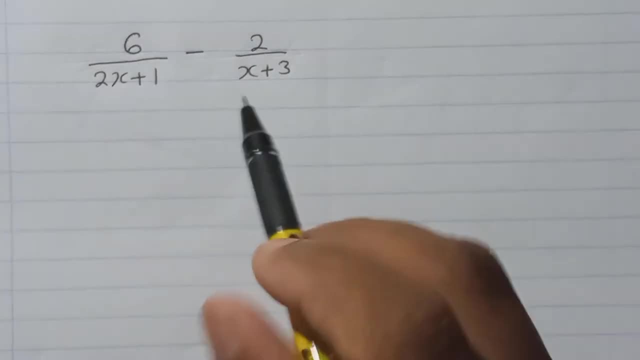 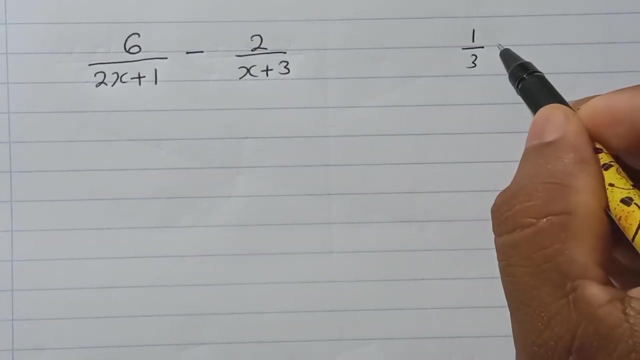 okay, think how to do this question. right, this is algebraic fraction, right, this is. you can think, like you know, when you have like normally like this kind of number, how we do, right, we make the same denominator, we can make same denominator to get the same denominator. what we do, this three. 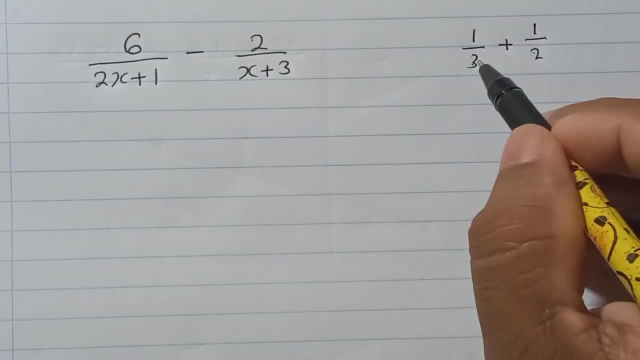 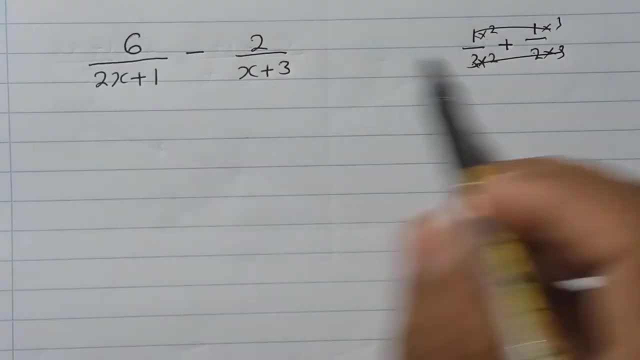 multiplied by this denominator, or make the lcm of this two somehow. so i will multiply by two here. so i also multiply by two. here i need to multiply by three. so here also multiply by three. now here six. here also six, like that. here also now. look here, try to understand what i did. this denominator. 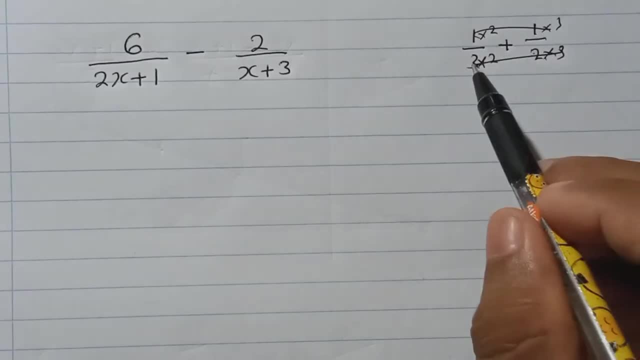 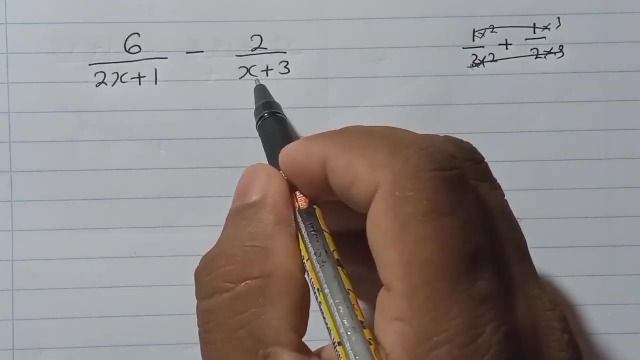 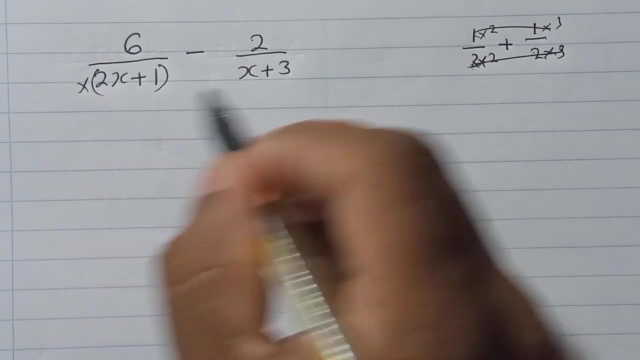 i multiply this one denominator, this denominator, i multiply this one denominator, like that. here also, i can multiply this denominator by this one, get the same denominator, can know. so i will multiply this denominator. okay, I will write here: x plus 3, this whole thing I need to multiply by this. that's why I put this: 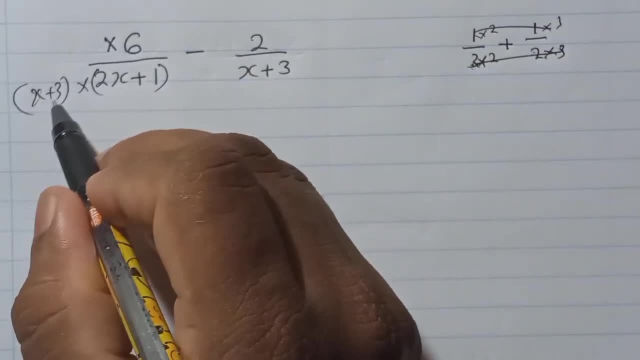 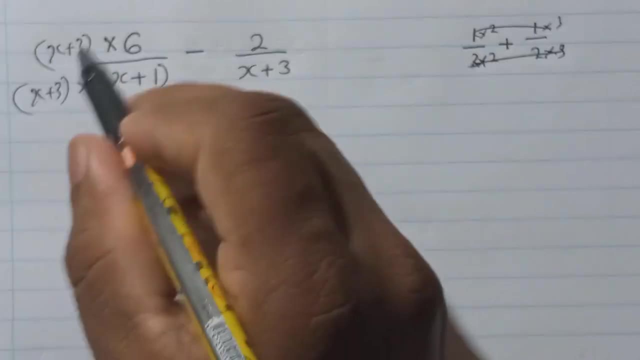 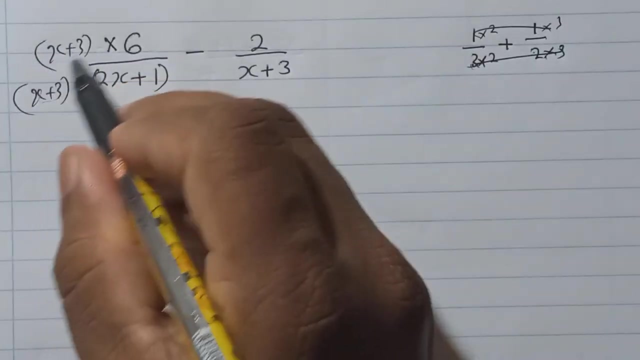 way right. and this 6 also I need to multiply by this one denominator that mean x plus 3 by x plus 3. right here I need to put bracket because 6 with this both. now this this denominator has two terms: x plus 3, that by that both you need to multiply this one. that's why I put inside bracket and. 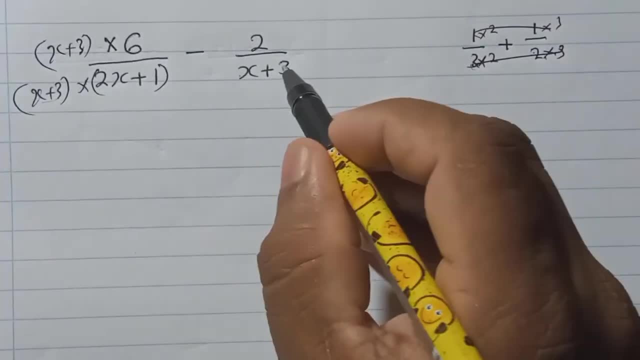 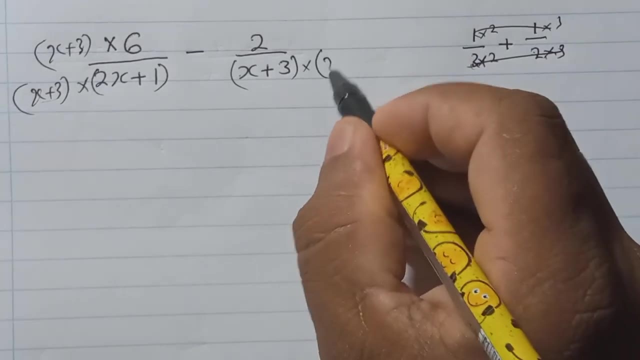 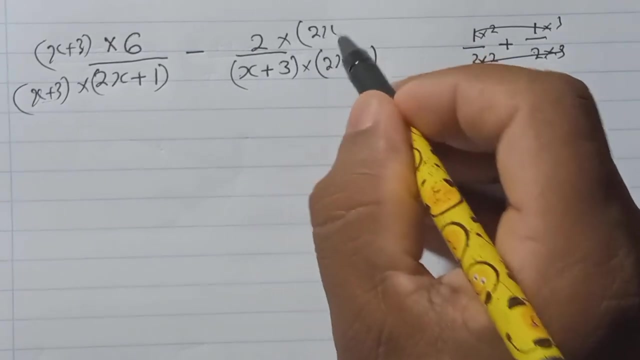 multiply by that. right here I need to multiply by this one, by this one denominator, this one denominator, by the 2x plus 1. here I need to multiply by 2x plus 1. so here also, in this numerator also, I need to multiply by 2x plus 1. that's why I put bracket right now. okay, now here. 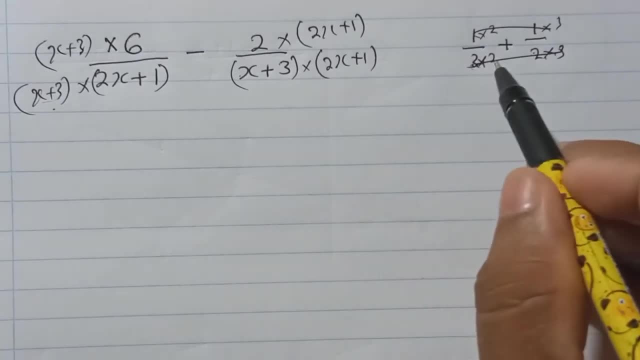 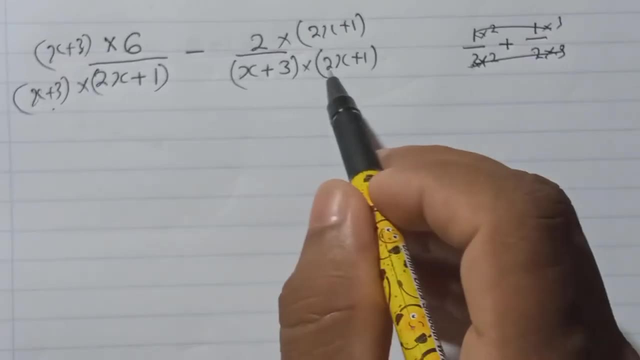 and here we have same denominator. you can see here like 3 into 2, 2 into 3, like that. here also we have same denominator: x plus 3 into 2x plus 1. here also x plus 3 into 2 x plus 1. so I need to write just that one rather. 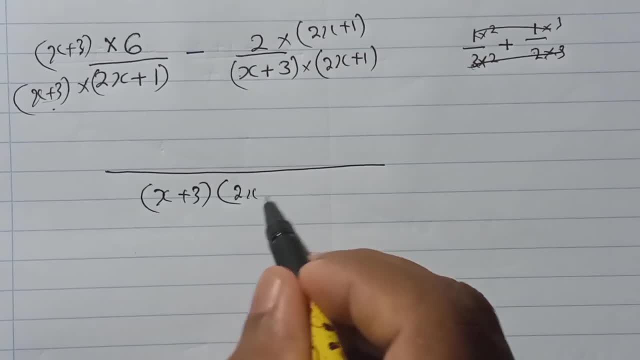 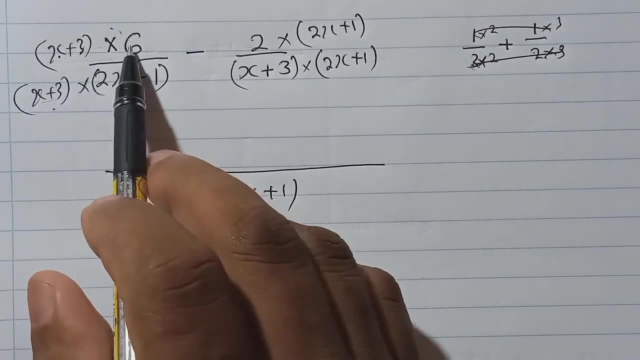 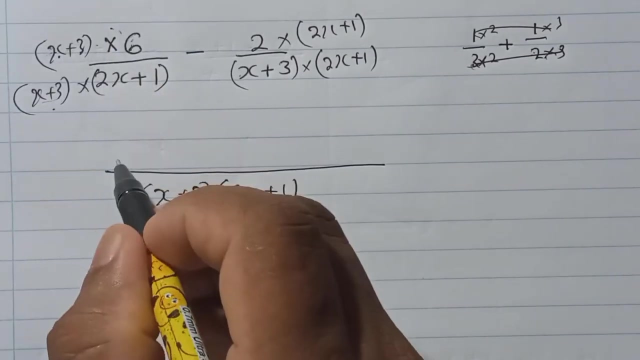 x plus 3 and here 2x plus 1, same denominator. now we have now in the after what you have. you have to do there by 6, you need to multiply this both, or by this: you need to multiply 6, so 6 into x it. 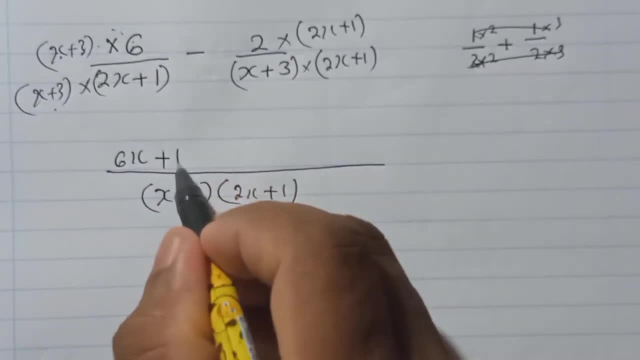 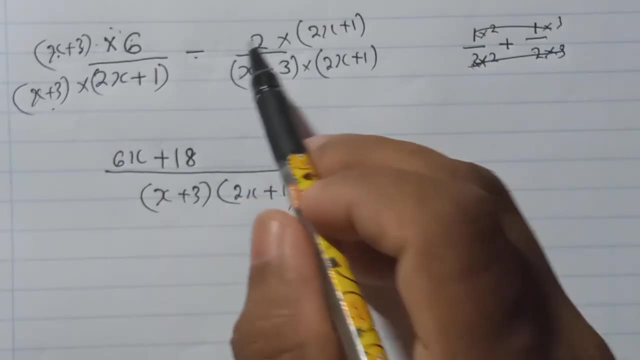 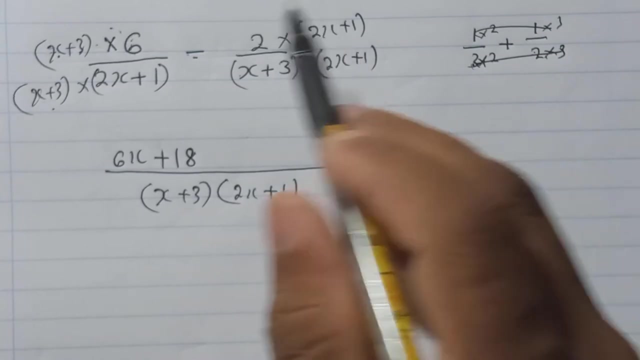 will be 6 x 6 into 3, it will be just 18. now here we need to multiply how here by minus 2. here- this is the very important thing, this sign thing belong to this: 2 right by minus 2. you need to multiply this both right by minus. 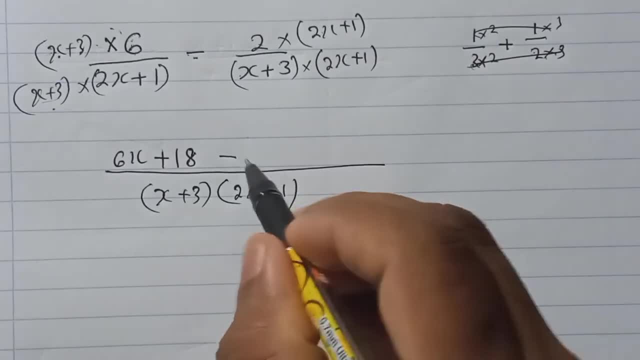 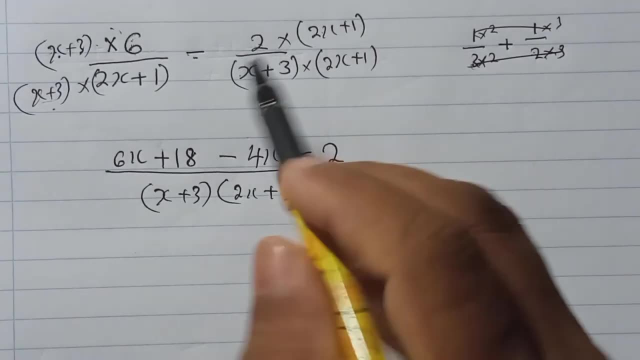 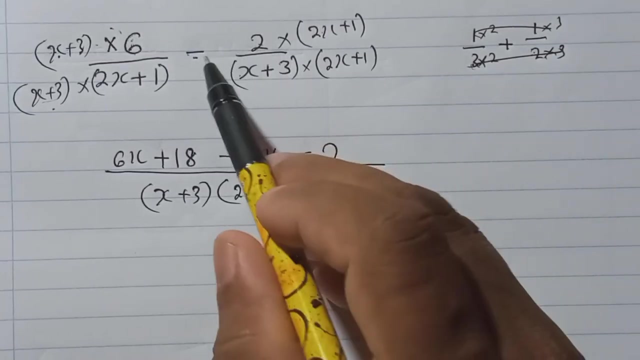 2. when you multiply here minus 2 into 2x, it will be minus 4x, and minus 2 into plus 1, it will be just minus 2, right? try to understand here very important thing: when you have this way, sometimes they will- you make single fraction like that here: minus sign between these two. 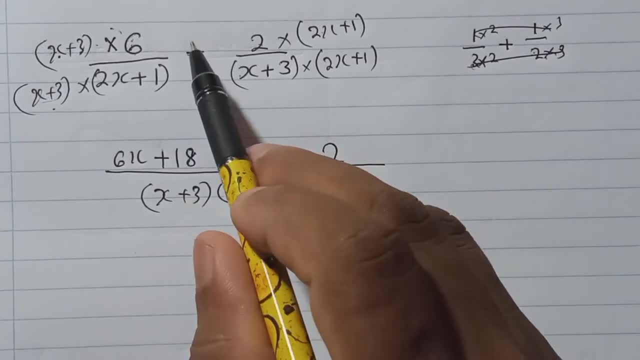 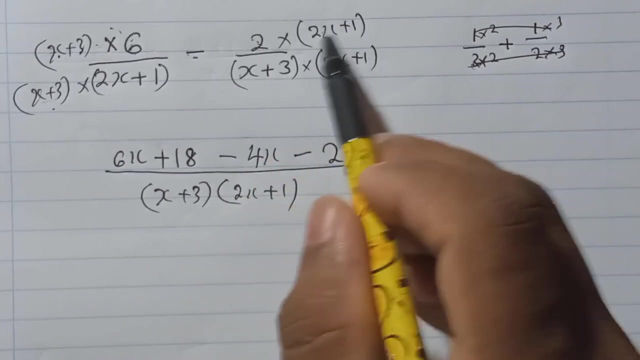 fraction when you have minus sign. very carefully, this minus thing belong to this number. by minus 2, whatever number you have here by minus sign belong to this number, things like that way. this sign belong to this, then with that sign, multiply this here. I multiply how minus 2 into this: no. 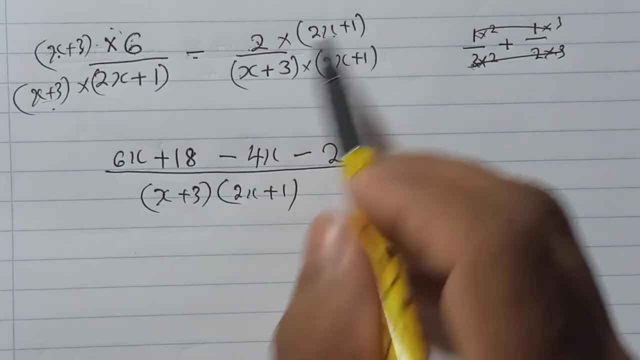 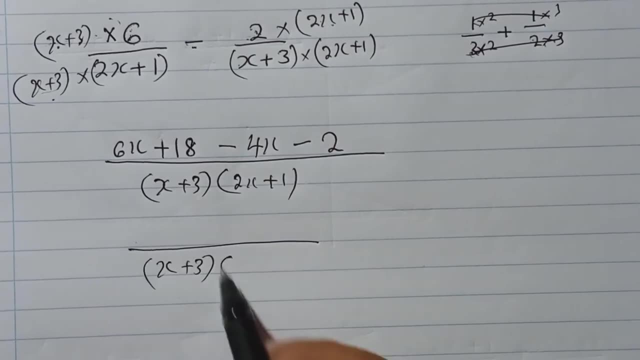 it's like that: if they are both equal, then you have minus 2 into this. no, it's like that, if they are half words, here 5 minus 5 into this, like that. okay, now what we have: here x plus 3 and here 2x plus 1. 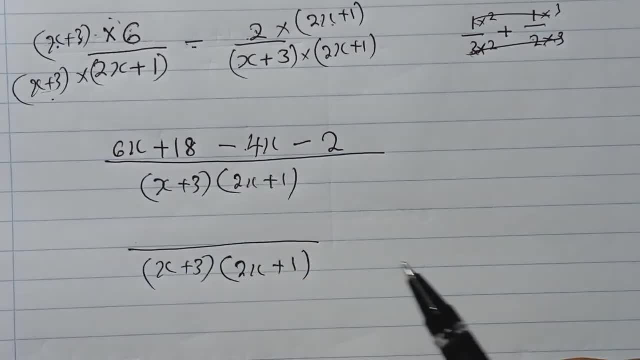 and 6x minus 4x. what the answer? 6x minus 4x. what answer? it's like them. so you can simplify it's. you can think: has 6 minus 4. like that you can think: 6 minus 4, me 2x and 18 plus 18 minus 2,. 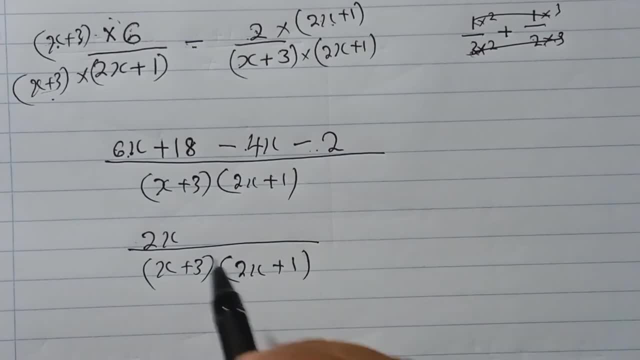 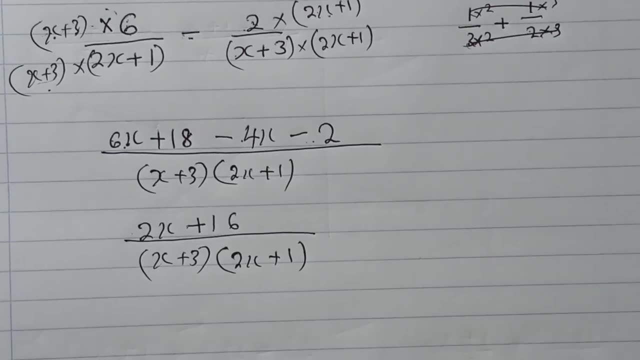 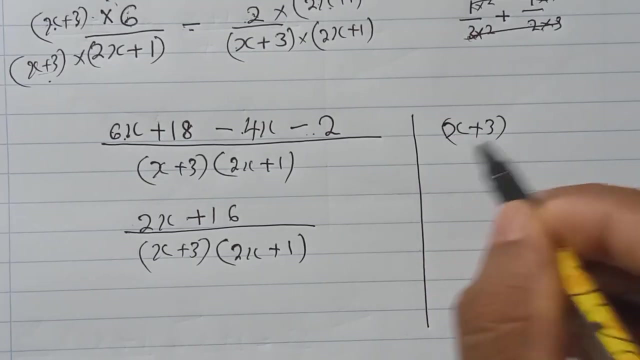 you can think: 18 minus 2, 18 minus 2 for the answer, it will be plus 16. so that's the answer. this is the some time. but here you can further simplify, right, this one also. we can multiply. you know, right now, if if i show you that also is you have already learned this also, but i will